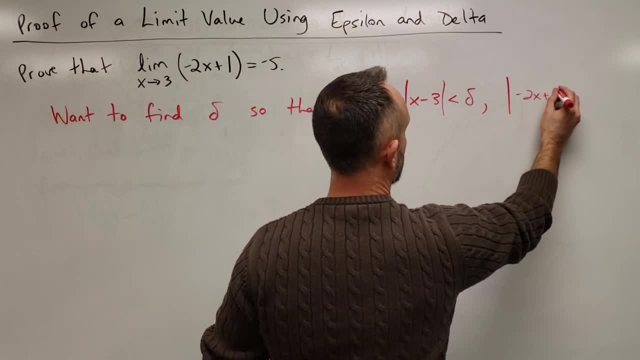 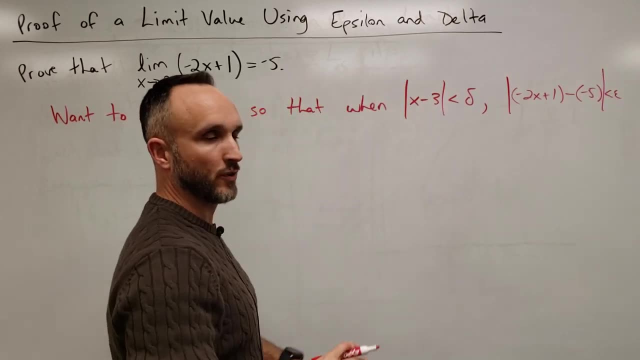 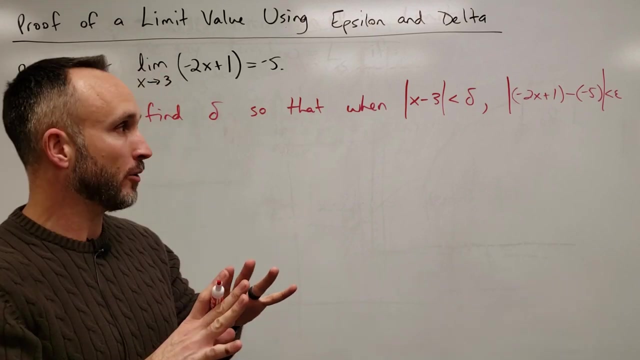 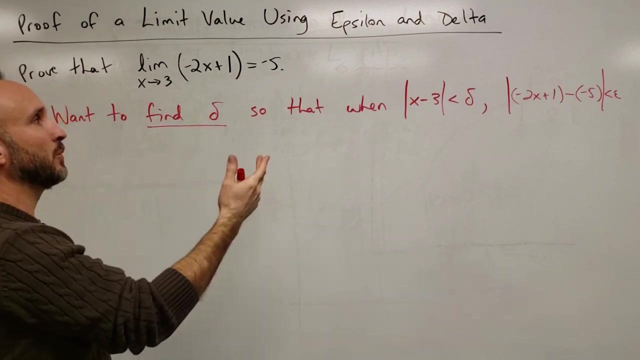 f of x is negative 2x plus 1, the distance between that and negative 5 is less than epsilon for any epsilon. So epsilon is given. We need to figure out delta. Okay, So this is our preliminary work. We need to. we need to find delta. We're going to do that first. Once we find delta, then we're going to go back and do the proof. Okay, So let's find delta. 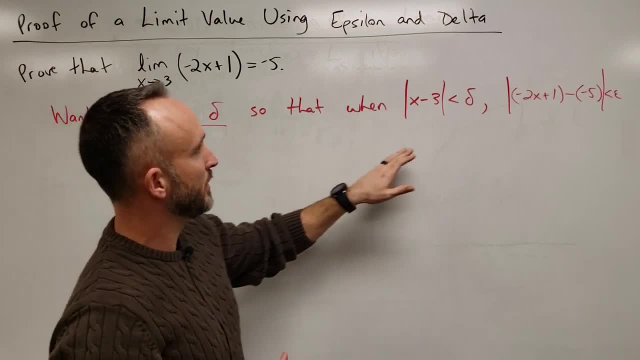 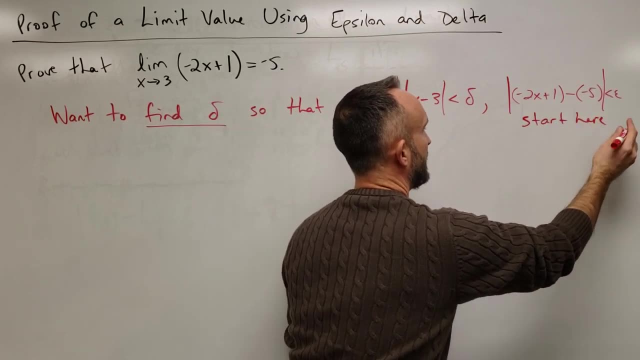 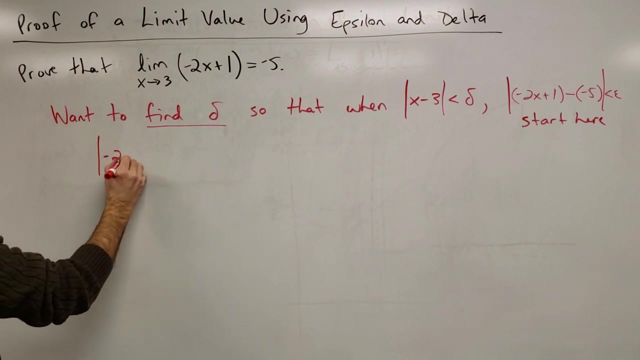 Okay, So let's find delta, But I want this epsilon statement to be true. Let's start here. Let's start with this and see if this can give us a hint as to what to choose delta to be. So let's let's take the absolute value of negative 2x plus 1, f of x minus l. the limit l is negative 5.. I want that to be less than epsilon. Okay, Let's clean it up, see what happens. and our goal is basically to find delta. 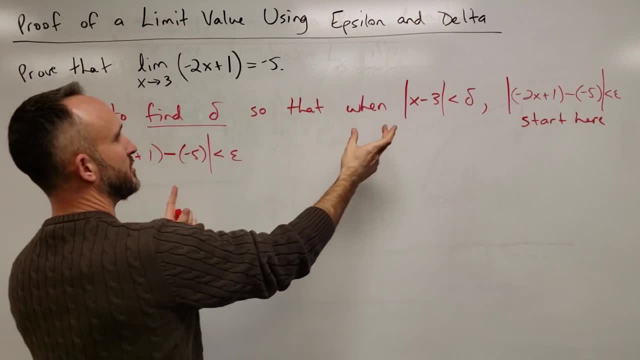 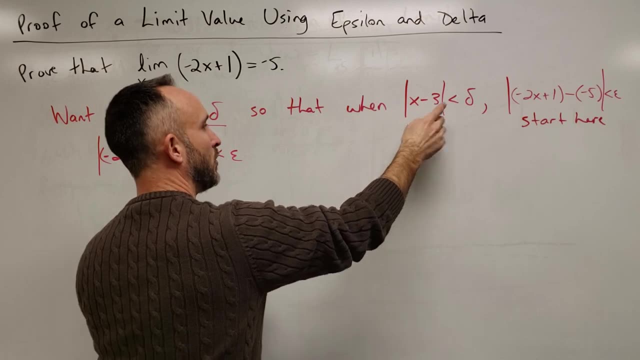 Really going to be. can I turn the absolute value into the absolute value of x minus 3?? Because if I can get x minus the absolute value of x minus 3 on the left side, whatever's on the right, that's going to be what I'm going to choose for my delta. 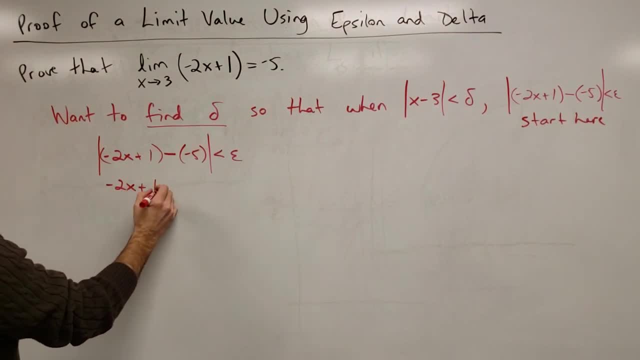 So negative 2x plus 1 minus negative 5 is the same thing as plus positive 5.. I want that less than epsilon. So I've got negative 2x plus 1 plus 5, which is plus 6, is less than epsilon. 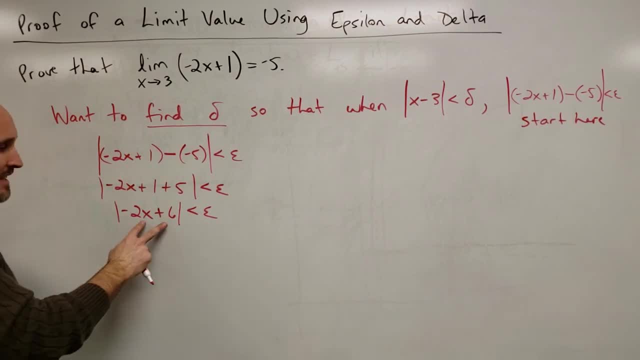 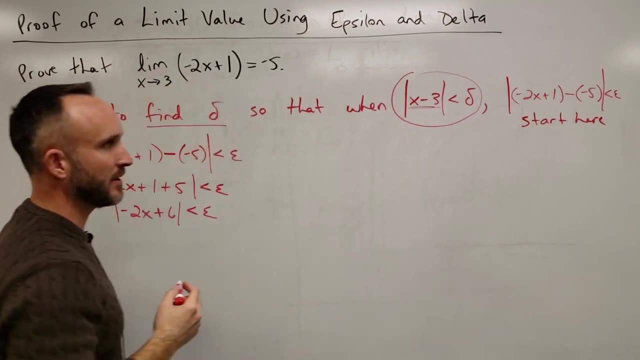 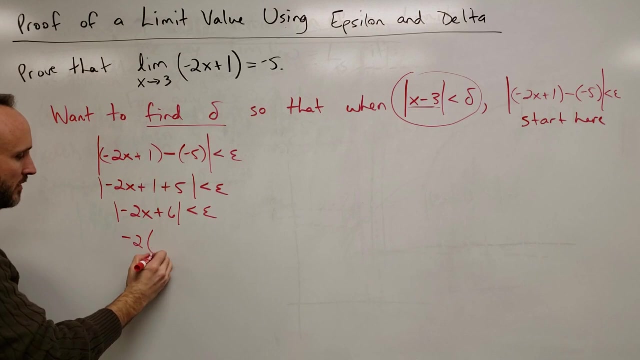 than epsilon. And then I look inside the absolute value and I compare it to what I want. I want this In particular: I want x minus 3 in the absolute value. So I notice what I can do here is I can factor this negative 2 out and that leaves positive x and negative 3.. Again. 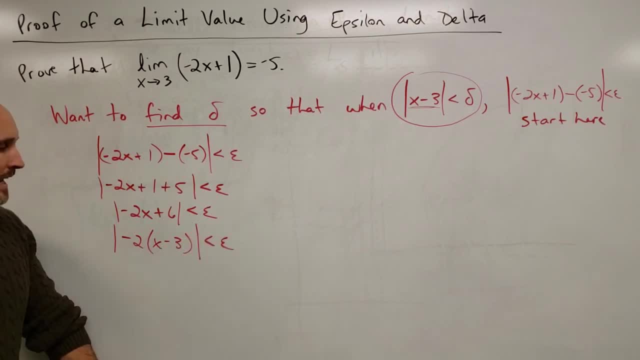 that's inside the absolute value. Now, the absolute value of a negative or a positive is the same. So what I can do here is I can say: well, this is the same thing as the absolute value of positive 2 times x minus 3.. It doesn't matter, right, Because a negative times this. 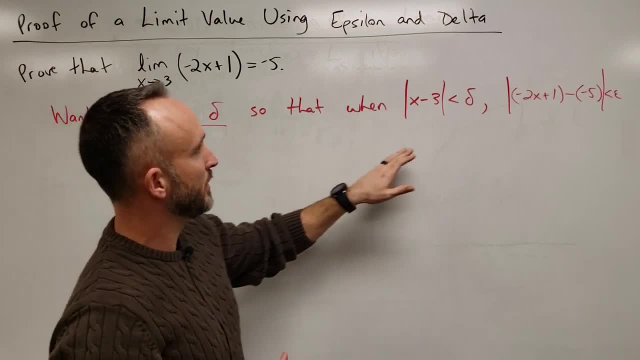 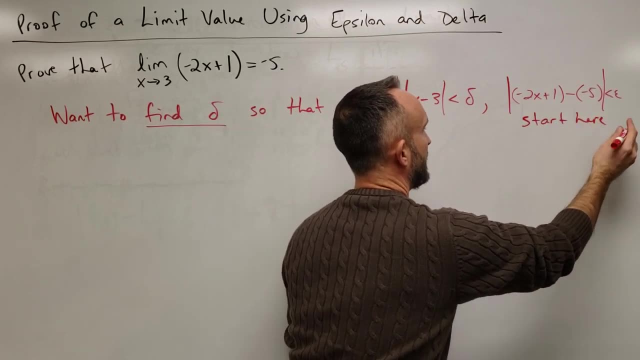 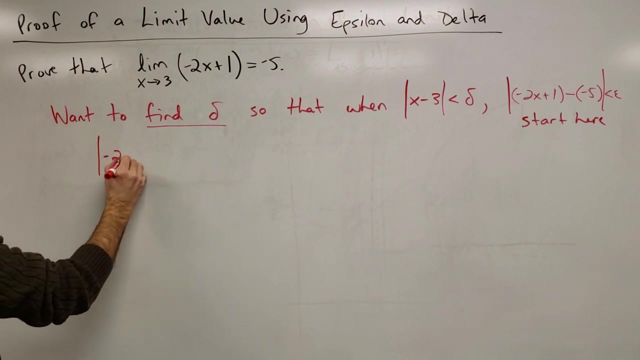 Okay, So let's find delta, But I want this epsilon statement to be true. Let's start here. Let's start with this and see if this can give us a hint as to what to choose delta to be. So let's let's take the absolute value of negative 2x plus 1, f of x minus l. the limit l is negative 5.. I want that to be less than epsilon. Okay, Let's clean it up, see what happens. and our goal is basically to find delta. 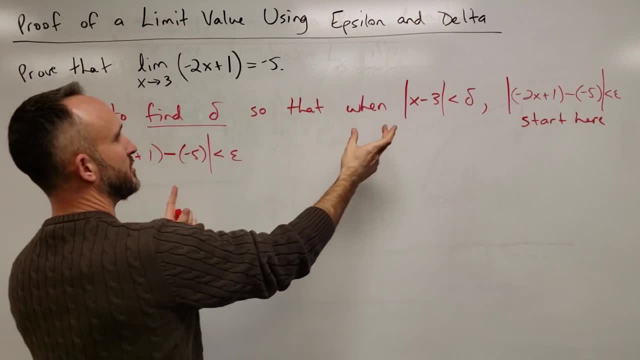 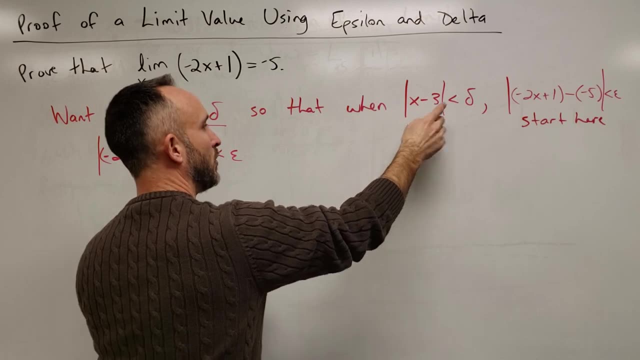 And I'm actually going to be. can I turn the absolute value into the absolute value of x minus 3?? Because if I can get x minus the absolute value of x minus 3 on the left side, whatever's on the right, that's going to be what I'm going to choose for my delta. 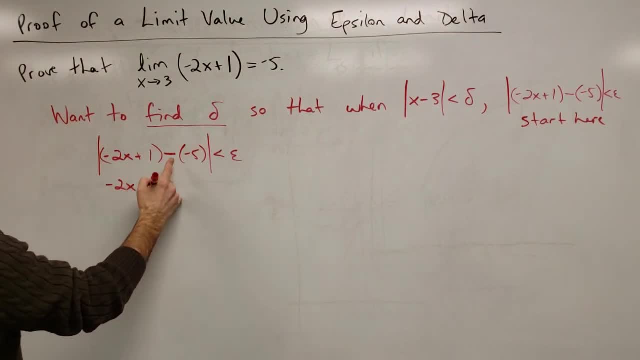 So negative 2x plus 1 minus negative 5 is the same thing as plus positive 5.. I want that less than epsilon. So I've got negative 2x plus 1 plus 5, which is plus 6, is less than epsilon. 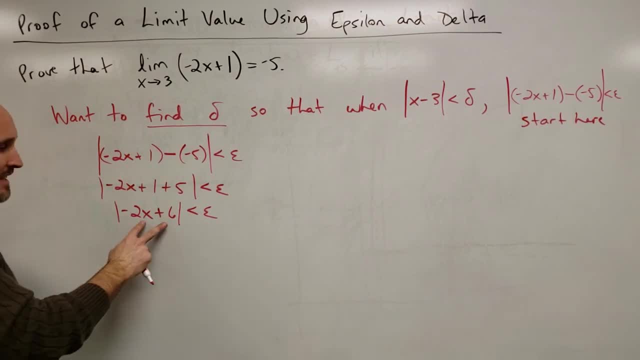 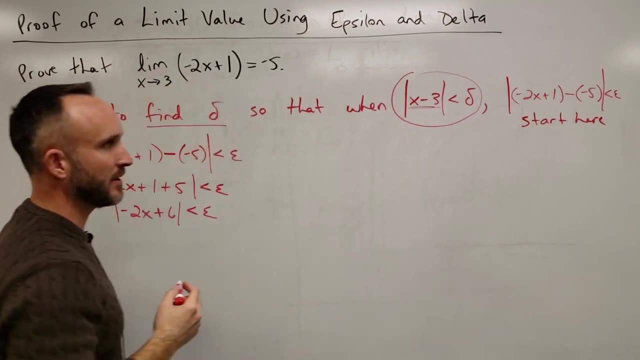 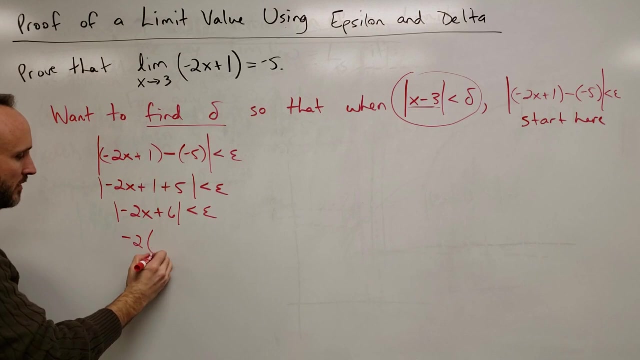 than epsilon. And then I look inside the absolute value and I compare it to what I want. I want this In particular: I want x minus 3 in the absolute value. So I notice what I can do here is I can factor this negative 2 out and that leaves positive x and negative 3.. Again. 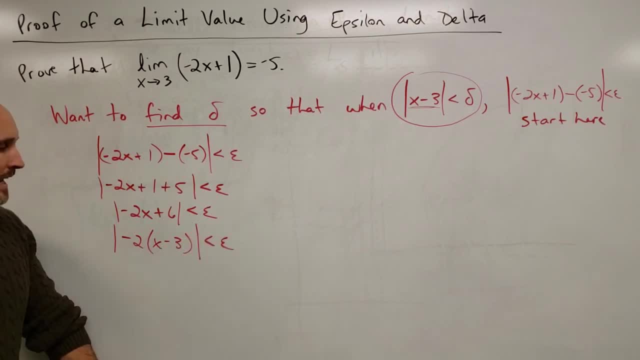 that's inside the absolute value. Now, the absolute value of a negative or a positive is the same. So what I can do here is I can say: well, this is the same thing as the absolute value of positive 2 times x minus 3.. It doesn't matter, right, Because a negative times this. 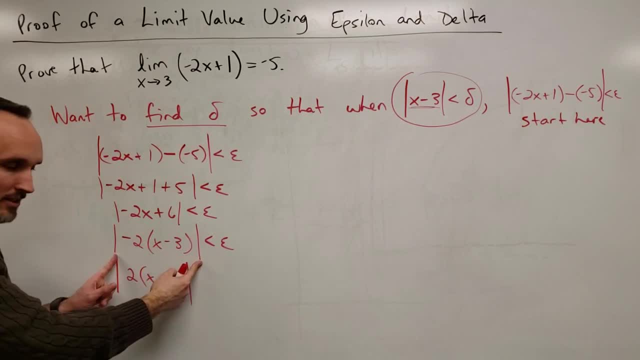 is going to be one value And when you take the absolute value it's going to be positive. Or you can do positive 2 times this and take the absolute value and still get a positive. Okay, And now the only barrier between this absolute value and what I want is this: 2.. 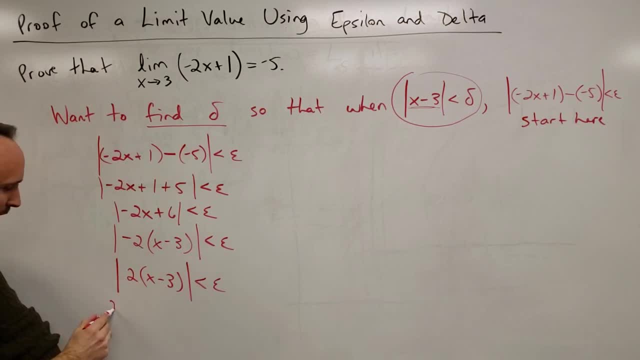 But since the 2 is positive, it's the same thing as multiplying by positive 2 outside of the absolute value. And that's the key: How do you factor and pull the constant out so that what remains is what you want? So you have to understand absolute value as well. 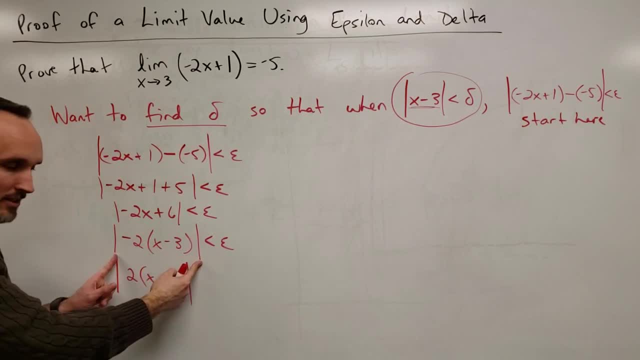 is going to be one value And when you take the absolute value it's going to be positive. Or you can do positive 2 times this and take the absolute value and still get a positive. Okay, And now the only barrier between this absolute value and what I want is this: 2.. 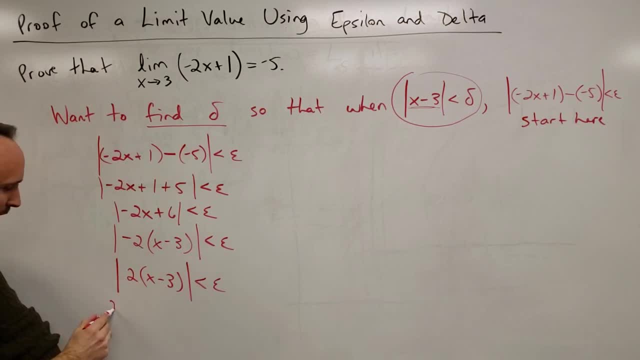 But since the 2 is positive, it's the same thing as multiplying by positive 2 outside of the absolute value. And that's the key: How do you factor and pull the constant out so that what remains is what you want? So you have to understand absolute value as well. 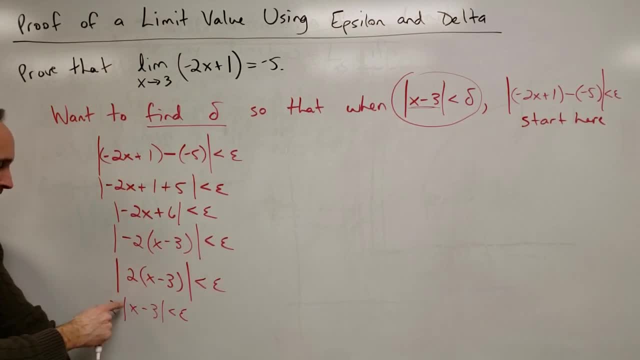 to understand. you can lose the negative And then, because this is positive, you want to multiply it by the positive 2, outside the absolute value. And now to get the absolute value by itself, it's very simple: Divide both sides by 2.. 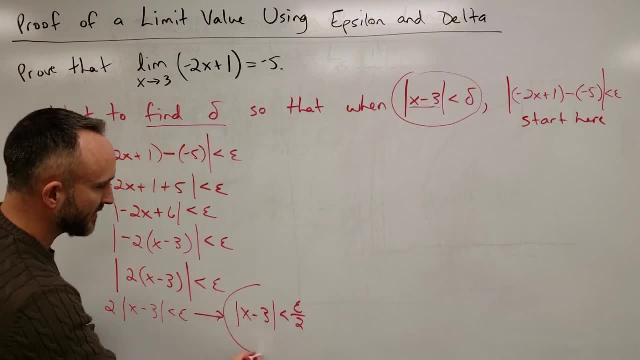 So what we're going to do is now: this statement is equivalent to this epsilon statement we started with, because we did it through a series of equivalent statements, And so we know that if this is true, that's going to be true, And so we're going to do this, And so we're. 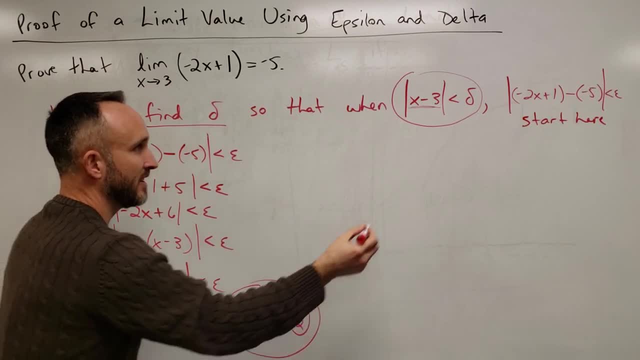 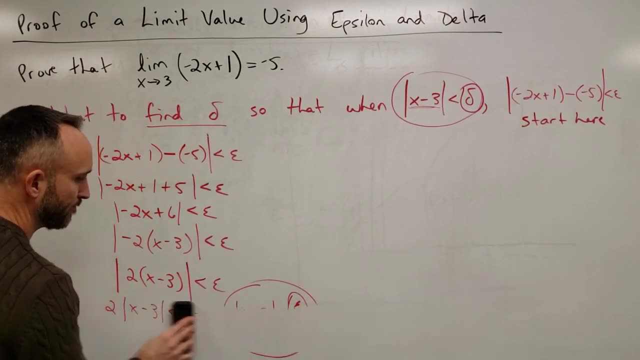 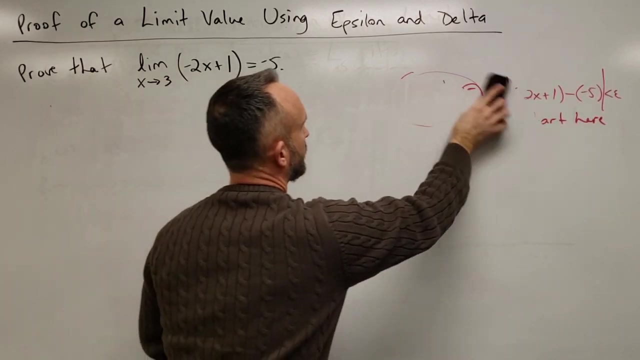 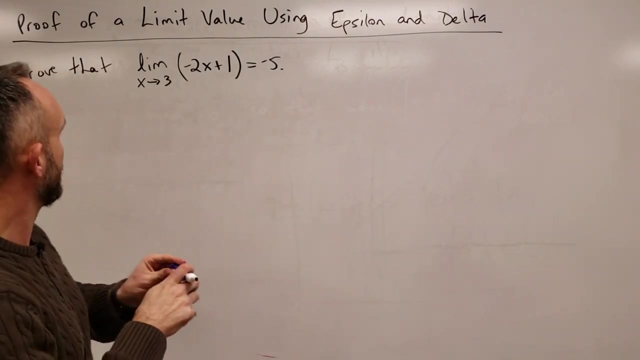 going to choose this to be the delta in our proof. So delta equals epsilon over 2.. Let's remember that. So here goes the proof. finally, We've done our preliminary work. We know our delta. So our proof is going to look like this: 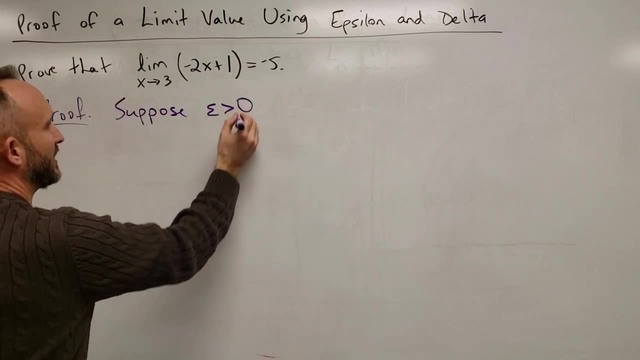 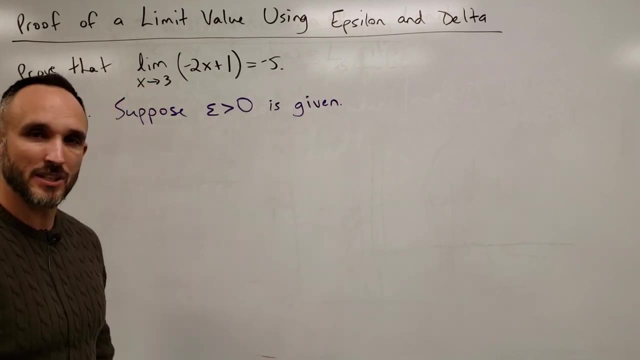 And so we have a meeting at Benchmark, right? How does the definition start? Well, you have to be given epsilon. So suppose epsilon greater than zero is given. Okay, Suppose epsilon greater than zero is given. Choose delta equal to epsilon over 2,, like we saw before. Okay, 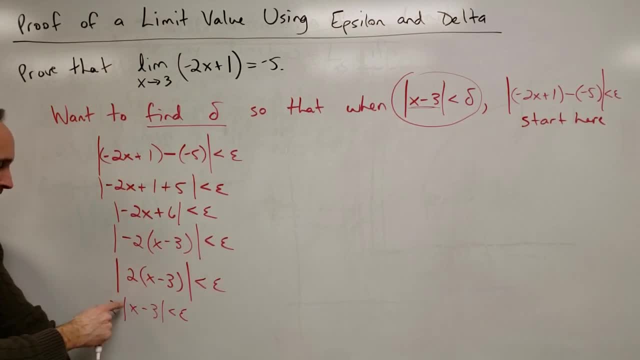 to understand. you can lose the negative And then, because this is positive, you want to multiply it by the positive 2, outside the absolute value. And now to get the absolute value by itself, it's very simple: Divide both sides by 2.. 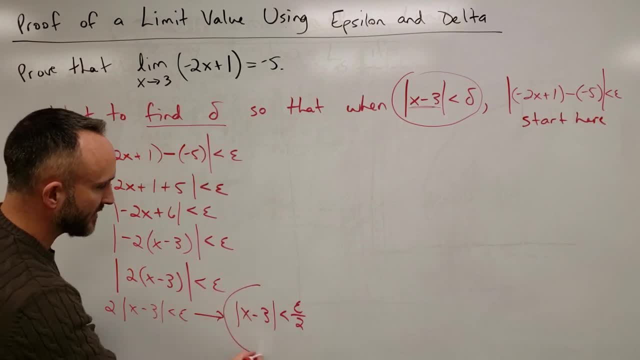 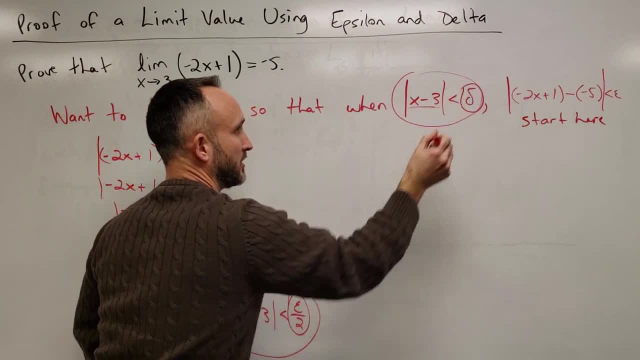 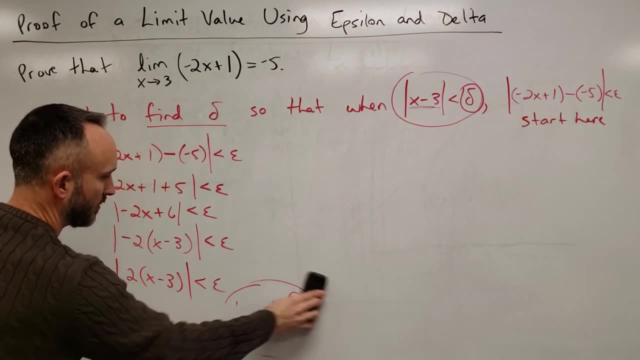 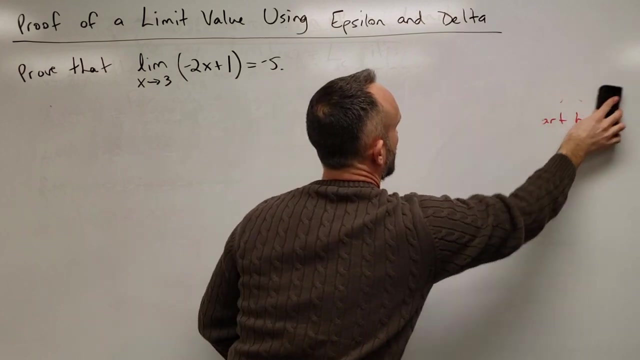 what we're going to do is we're going to choose this to be the delta in our proof. So delta equals epsilon over 2.. Let's remember that. So here goes the proof. finally, We've done our preliminary work. We know our delta. 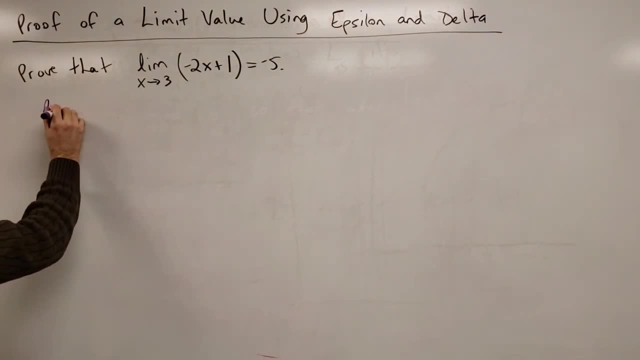 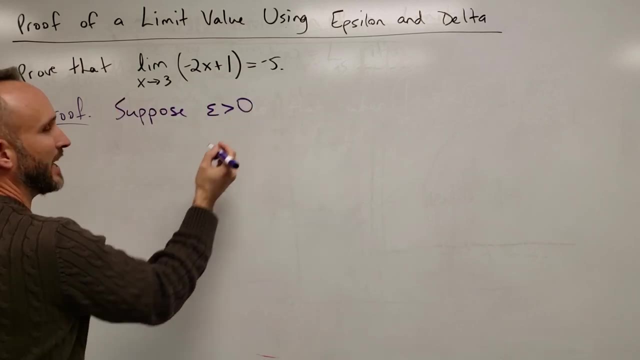 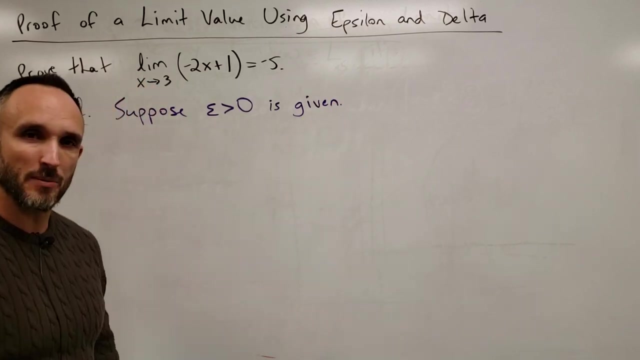 So our proof is going to look like this. right, how does the definition start where you have to be given epsilon? so suppose epsilon greater than zero is given. okay, suppose epsilon greater than zero is given, choose delta equal to epsilon over two, like we saw before. okay. 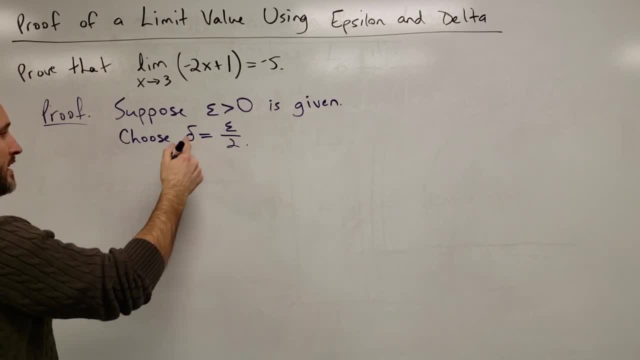 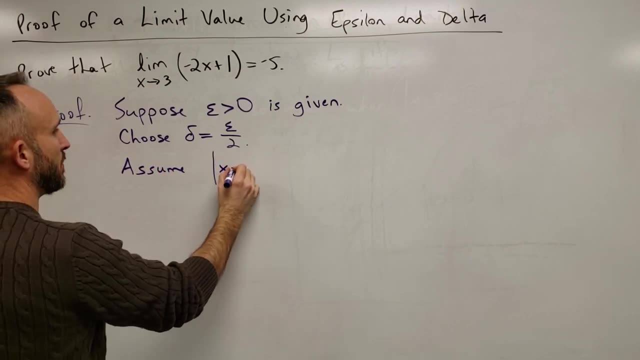 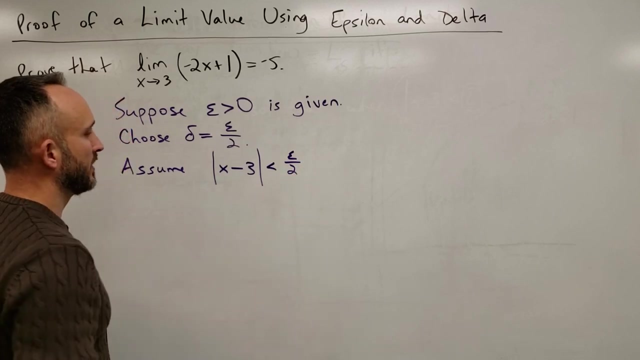 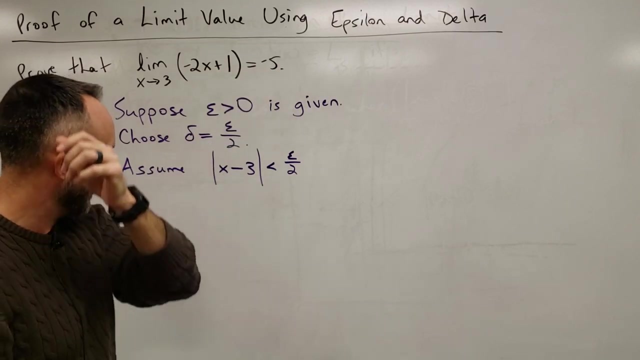 and what we're going to do is now. the definition says that if the absolute value of x minus three is less than delta, which is epsilon over two, if that's true, then the absolute value of negative 2x plus one minus negative five should be less than epsilon, right? 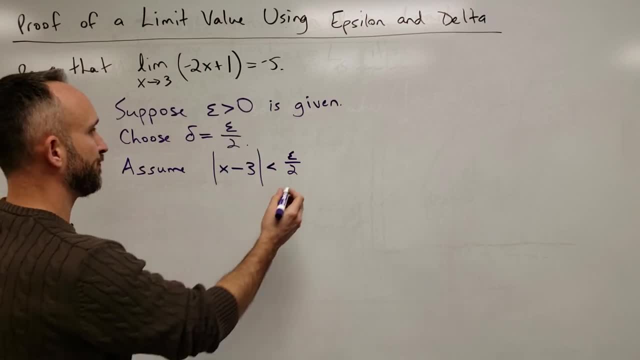 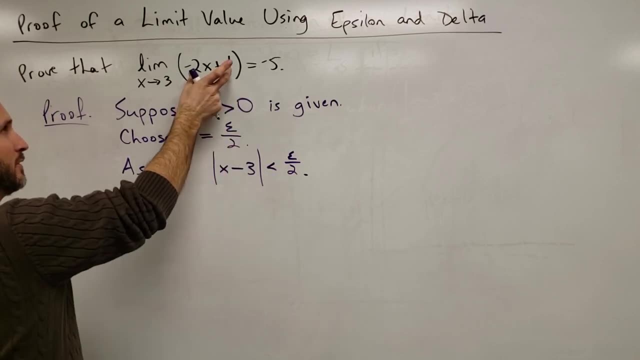 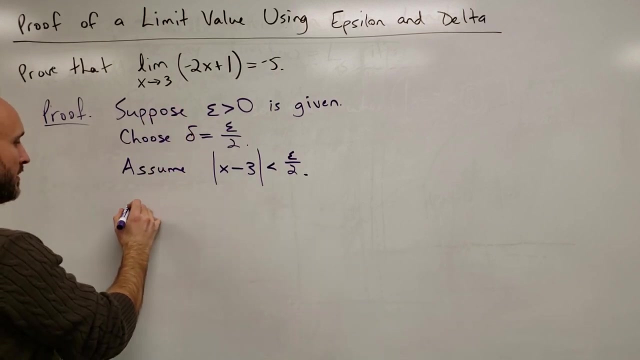 so that's what we're going to look at now. so assume this is true. okay, we want to. because of this, we want to be able to state that the absolute value of this function minus negative five is less than epsilon. so let's examine so now, the absolute value of negative 2x plus one. 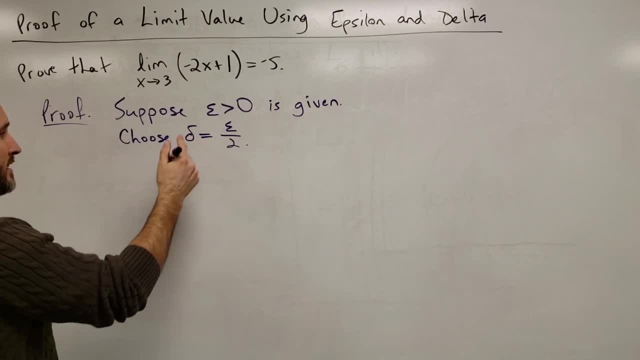 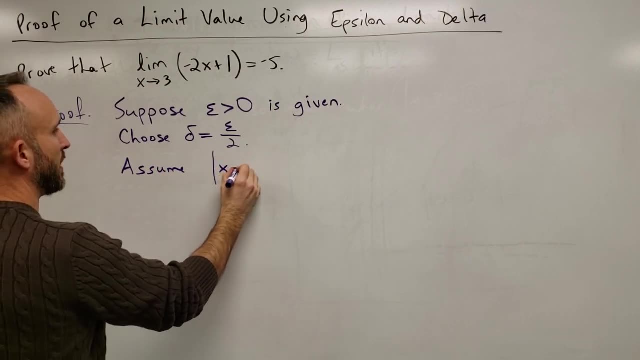 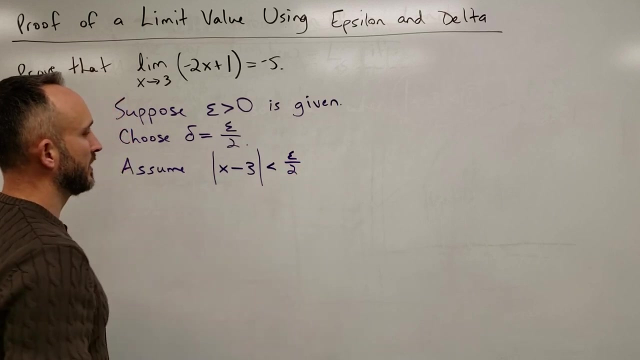 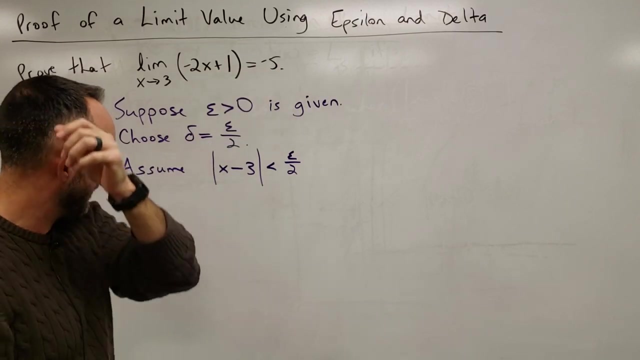 and what we're going to do is now. the definition says that if the absolute value of x minus 3 is less than Delta, which is epsilon over 2, if that's true, then the absolute value of negative 2x plus 1 minus negative 5 should be less than epsilon. right? so that's what we're going to look at now. 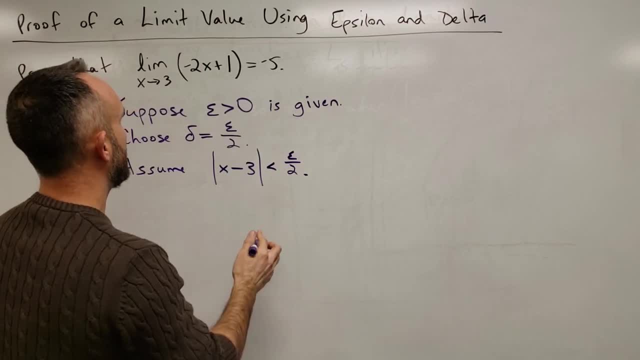 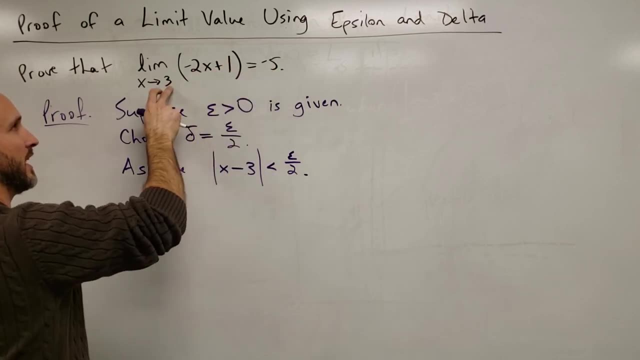 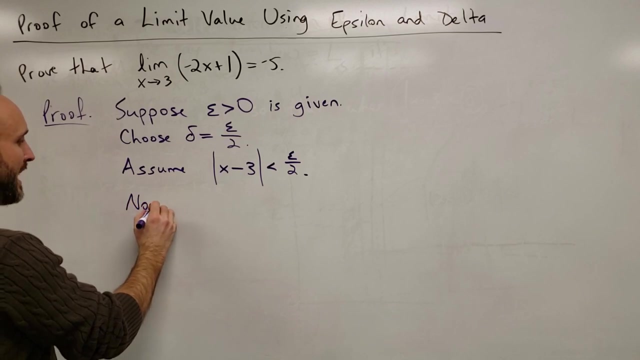 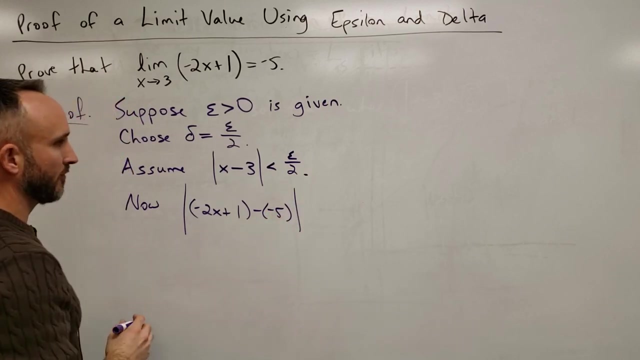 so assume this is true. we want to. because of this, we want to be able to state that the absolute value of this function minus negative 5 is less than epsilon. so let's examine so now. the absolute value of negative 2x plus 1 minus negative 5 equals the absolute value of negative. 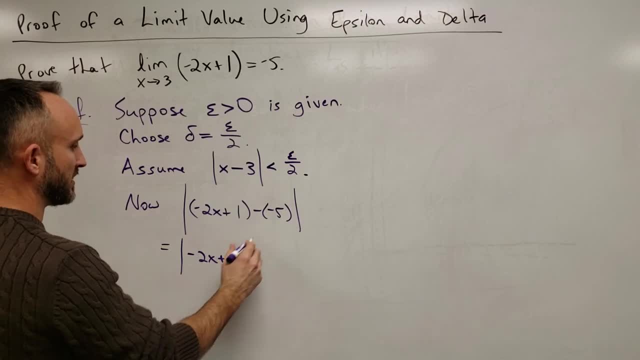 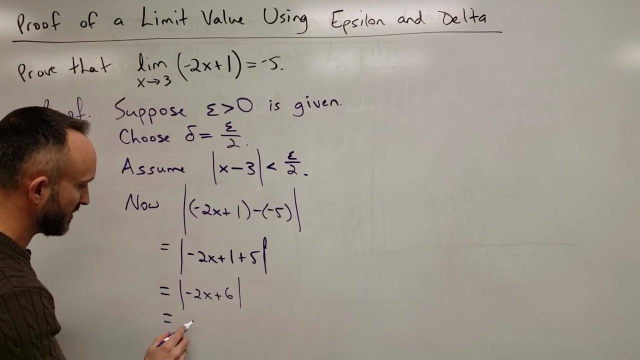 2x plus 1 plus 5- I know this work is familiar. we had to do a lot of the same work in our preliminary setup to find our Delta equals the absolute value of negative. 2x plus 6, which is the same thing as the absolute value of negative. 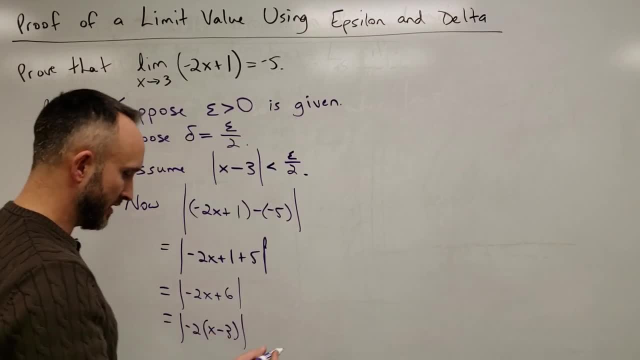 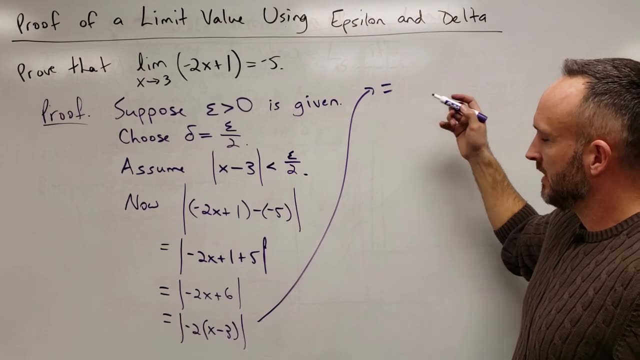 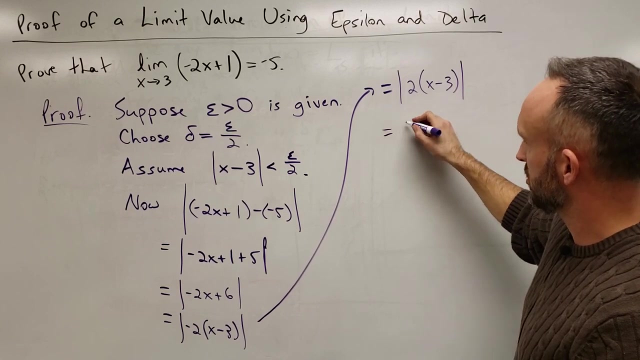 2 times the quantity X minus 3. let's come over here. if I had regular notebook paper, I'd work vertically. equals the absolute value of 2 times X minus 3, which equals- pull the 2 out- 2 times the absolute value of X minus 3. and now this: 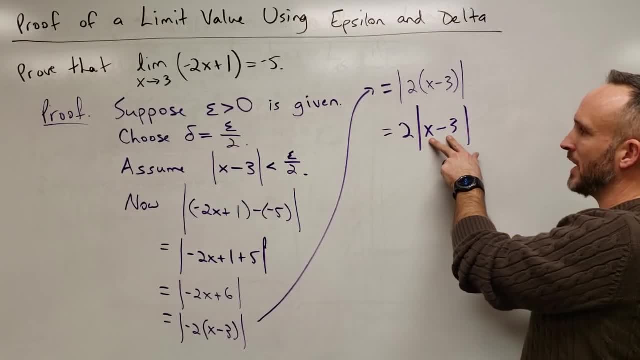 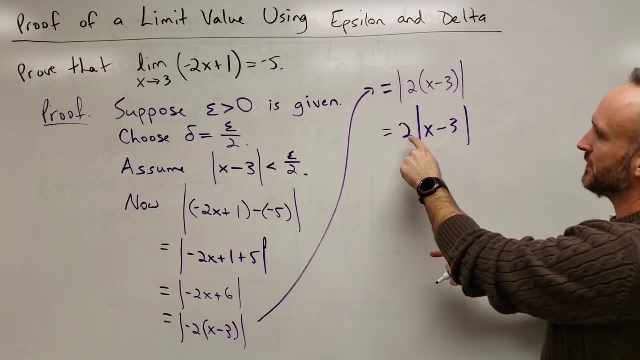 is where it's different. what do we know about the absolute value of X minus 3? the absolute value of X minus 3 is less than epsilon over 2, so that means if I take 2 times this positive number, it's going to be less than 2 times. 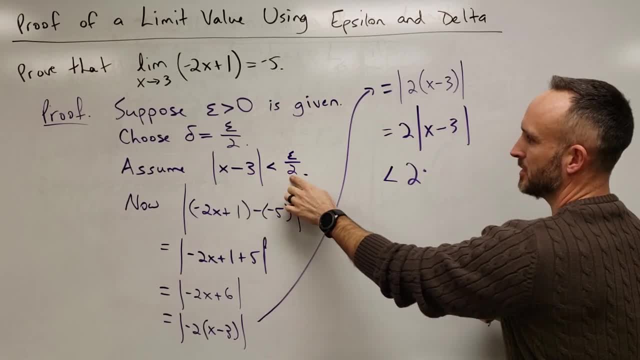 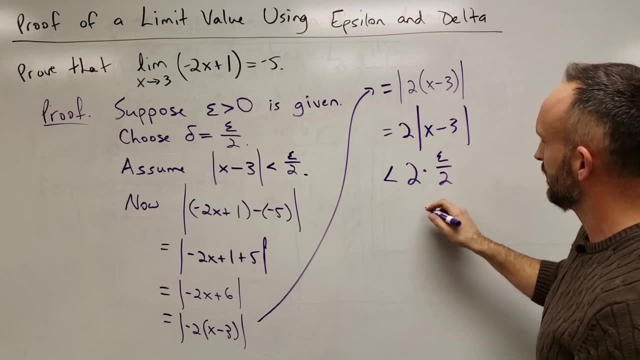 negative: 2x plus 1 plus 5, Well, the absolute value of x minus 3 is less than epsilon over 2, so this product is going to be less than the product of 2 and epsilon over 2,, which equals epsilon. 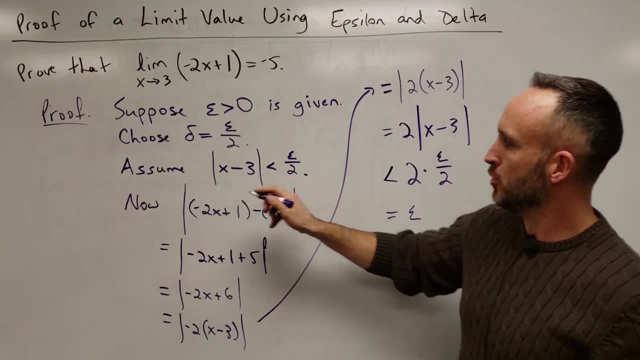 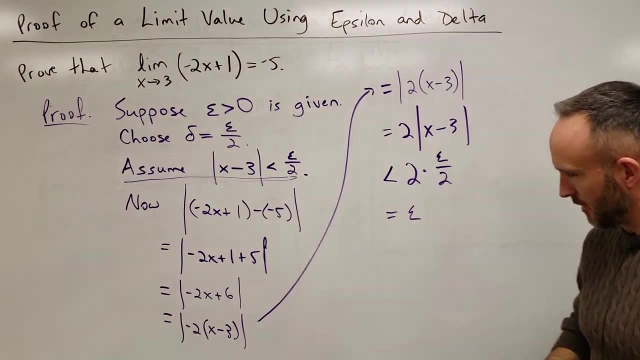 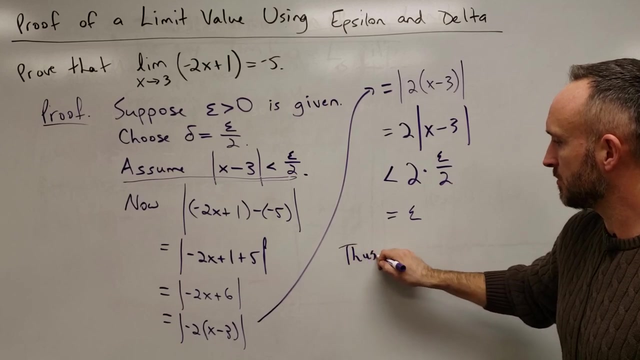 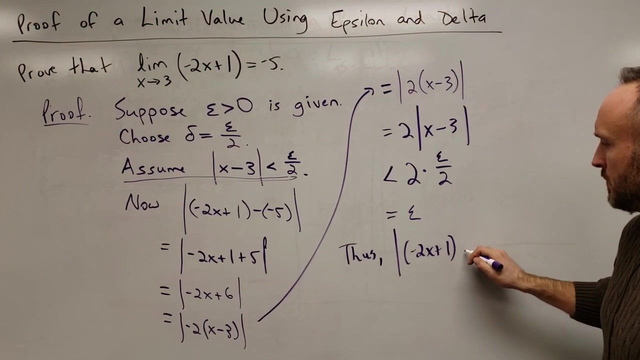 Okay, so let's go back. We assumed the delta statement. We assumed that the absolute value of x minus 3 is less than this delta epsilon over 2.. And we concluded thus: let's put it all together now. Thus, this guy here, the absolute value of negative 2x plus 1 minus negative 5,. 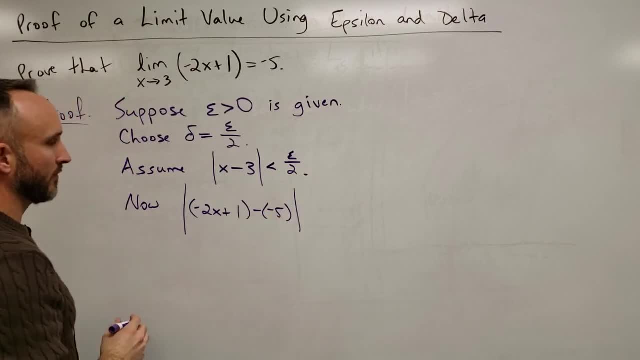 minus negative five equals the absolute value of negative two x plus one plus five. i know this work is familiar. we had to do a lot of the same work in our preliminary setup to find our delta equals the absolute value of negative two x plus six, which is the same thing as the absolute value of negative two times the quantity. 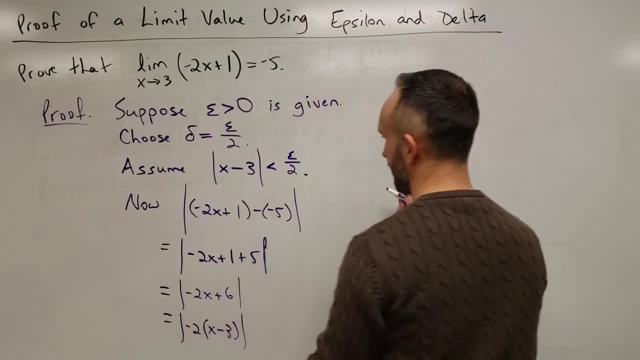 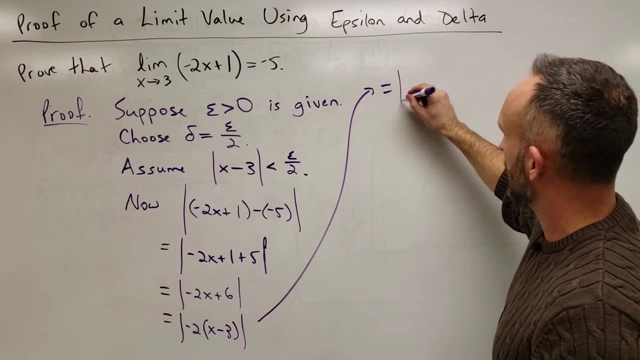 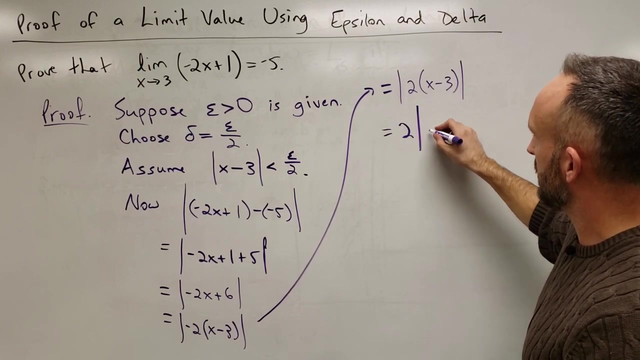 x minus three. let's come over here. if i had regular notebook paper, i'd work vertically- equals the absolute value of two times x minus three minus three, which equals- pull the two out, two times the absolute value of x minus three. and now this is where it's different. 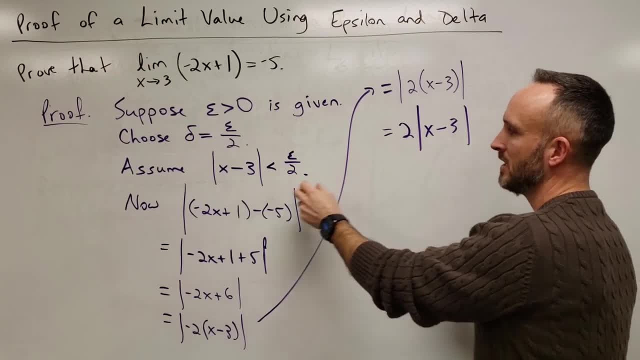 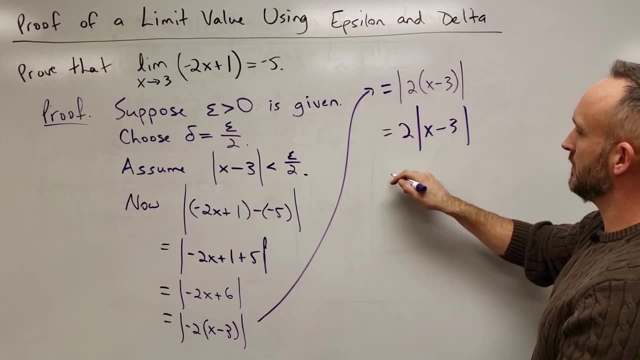 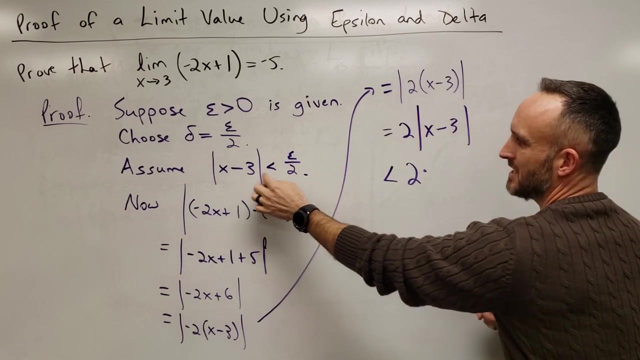 what do we know about the absolute value of x minus three? the absolute value of x minus three is less than epsilon over two. so that means if i take two times this positive number, it's going to be less than two times. well, the absolute value of x minus three is less than epsilon over two. so this: 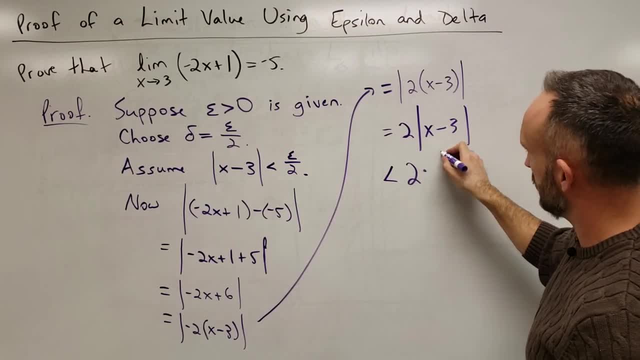 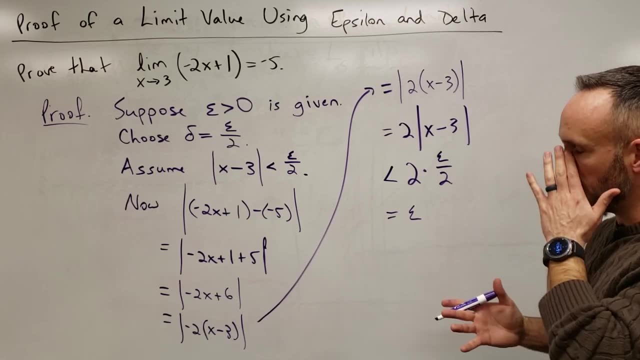 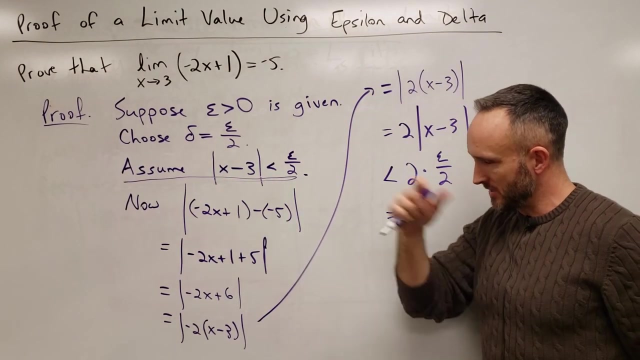 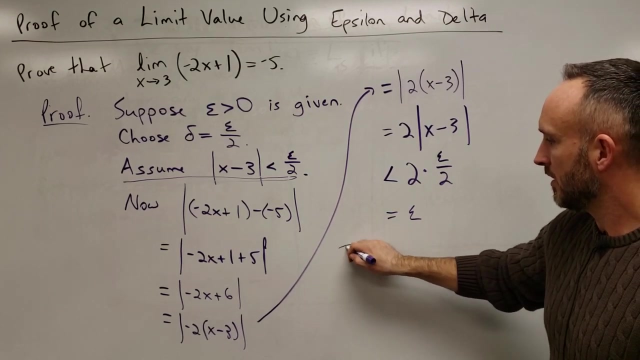 this product is going to be less than the product of two and epsilon over two, which equals epsilon. so let's, let's go back. we assumed the delta statement, we assumed that the absolute value of x minus three is less than this delta epsilon over two, and we concluded: 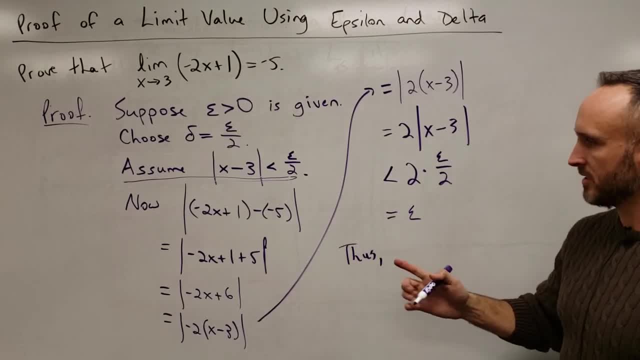 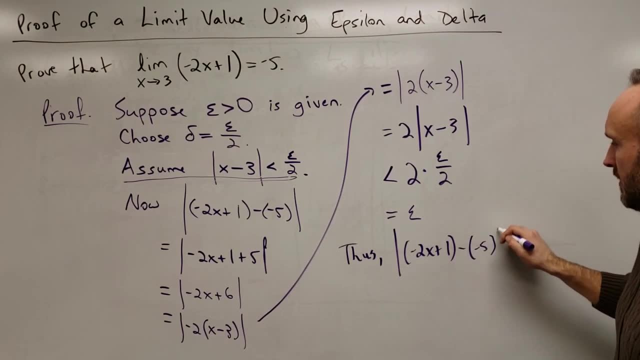 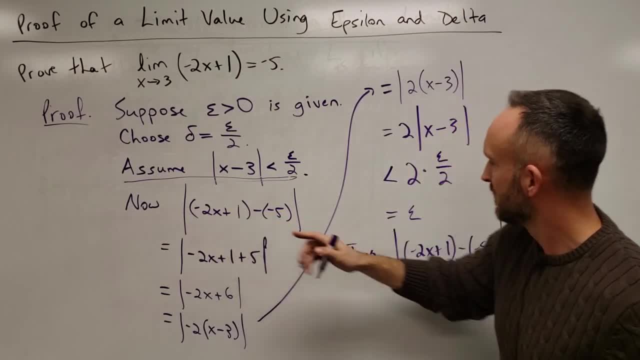 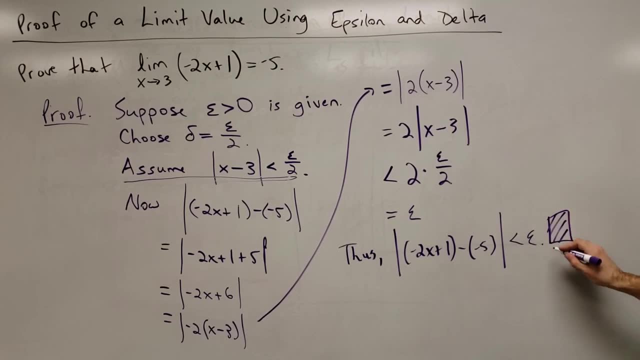 so, in other words, the original expression is less than epsilon, and that's the end of the proof, because we proved that if we assume this is true, then that led us to conclude that this is true and that's what the definition of the limit says has to be true. 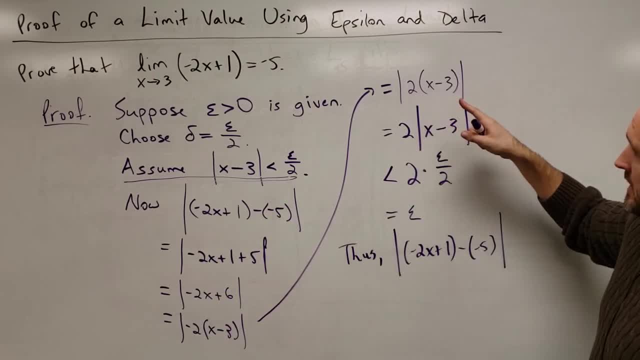 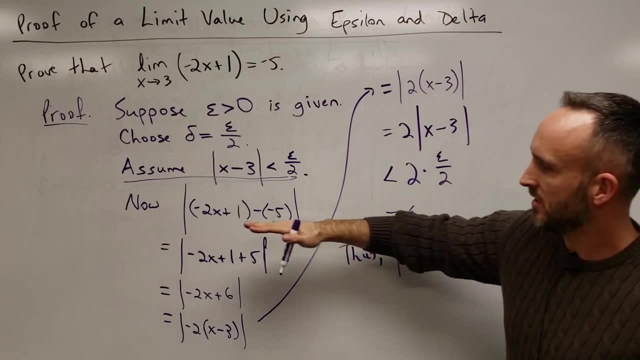 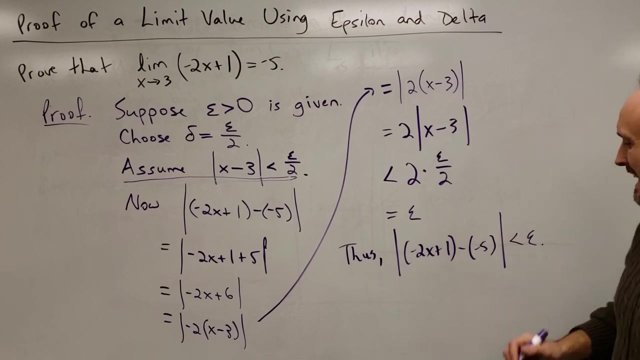